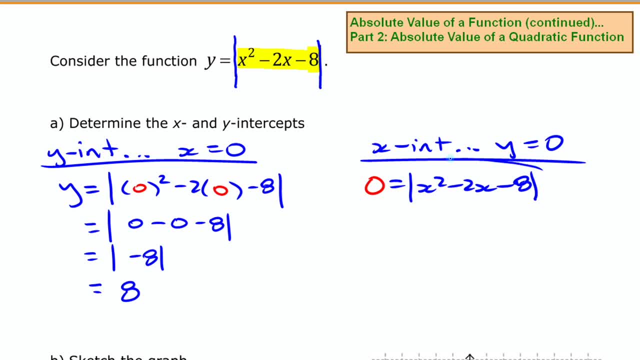 and solve this Now. as you've seen before, if we have absolute value of something equals 0, then the only way that that can work is if that something, in other words this, without the absolute value of brackets- has to equal 0. What that means is the x-intercepts of this absolute value function are going to be the 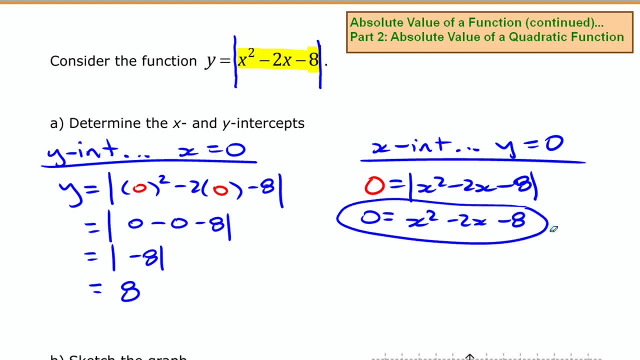 same as the x-intercepts of the original quadratic function which we'll see in a moment graphically Sketch the graph of the thing. Easiest way to solve this one is to factor. This one does factor. We have x plus 2, x minus 4, or in other words our x-intercepts. here are 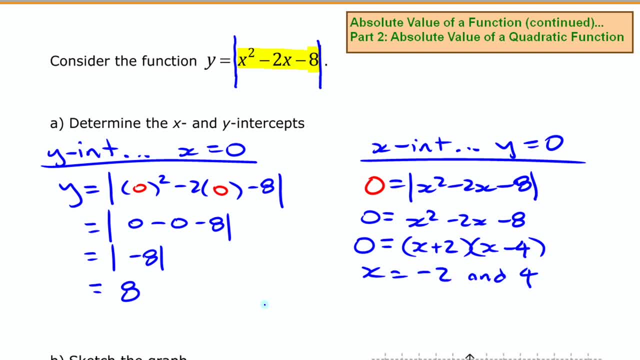 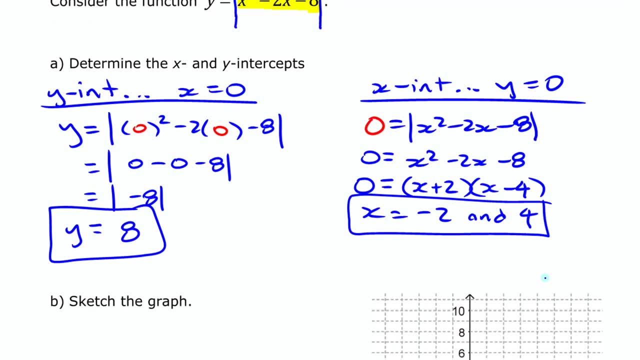 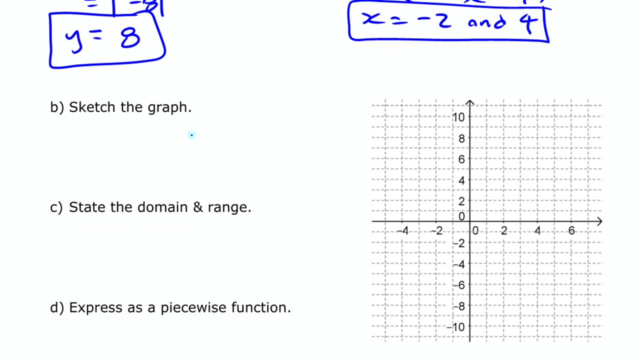 negative, 2 and 4.. All right, so we have a y-intercept of 8 and x-intercepts of negative, 2 and 4.. So we're going to try and sketch the graph of this thing here. We're going to use the strategy I described before. We're going to use x squared minus 2 x. 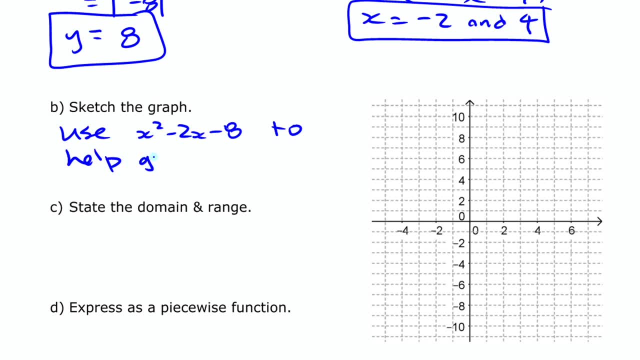 minus 8 to help graph absolute value of x squared minus 2, x minus 8.. So we're going to first think about this. We already know the x-intercepts. The x-intercepts are negative, 2 and 4.. Those do not change This and this. 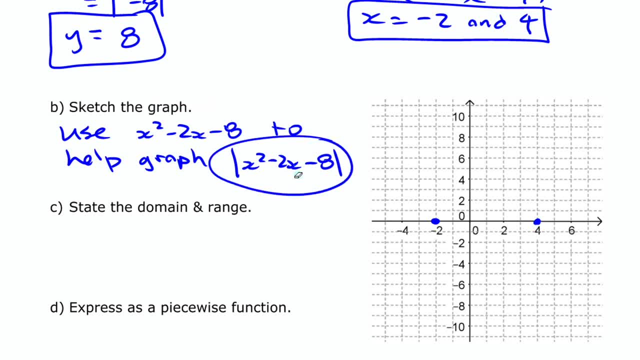 have the same x-intercepts So we can graph those on there. We did see that the y-intercept of the new function is going to be positive 8 up here, but without those absolute value brackets it would have been negative 8.. So the original quadratic that we have here would: 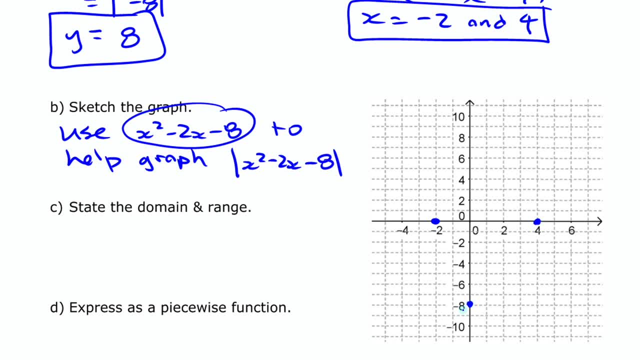 have had a y-intercept of negative 8. Now you can use a little bit of logic here. If you know that these are the two x-intercepts, you know that the axis of symmetry and the vertex have to be halfway in between there, So halfway in between there. 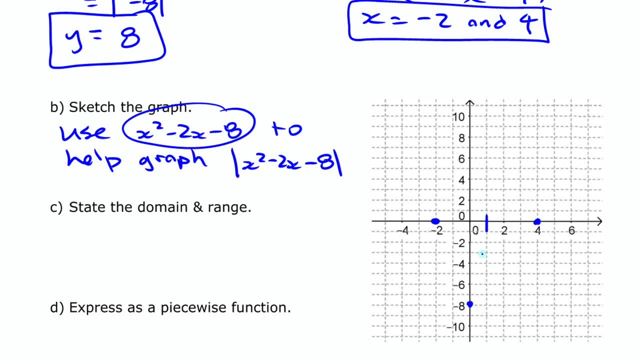 is actually 1.. So that's going to be the axis of symmetry. If you want to use that axis of symmetry to help with the graph, if you know this point and you know it's symmetric, you can also use that idea to tell you that this is also going to be a point on that graph. 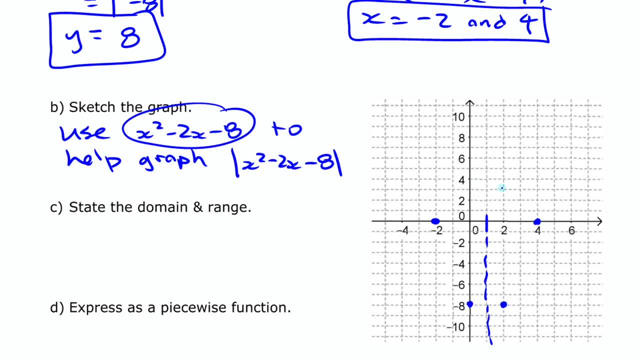 And you know that since that's going to be the vertex, you could substitute that value 1 into here to tell you what that vertex is. So if I put a 1 in there, in other words if I say 1 squared minus 2 times 1 minus 8, this is going to give me 1 minus 2 minus 8, which 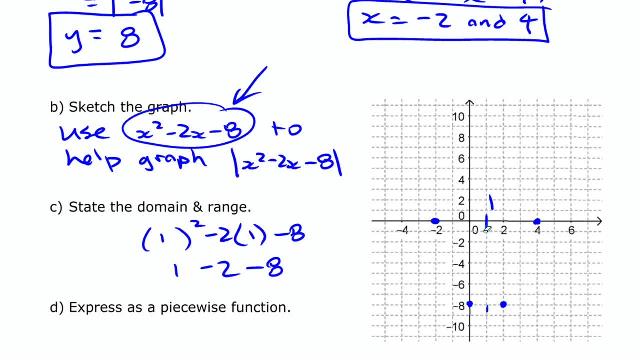 is actually negative 9, which is right here. That's probably enough to get the shape of this thing right. If you know the pattern in points there of that, you could actually probably also say that those two points are on there. But just for what we're doing here that's not absolutely. 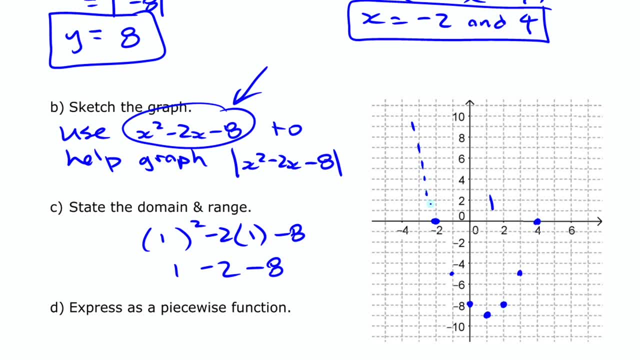 necessary. So we have a graph that looks something like this. That's the original function, more or less Okay. I haven't worried about any other points there other than the ones I already plotted there, But that is that original quadratic function. 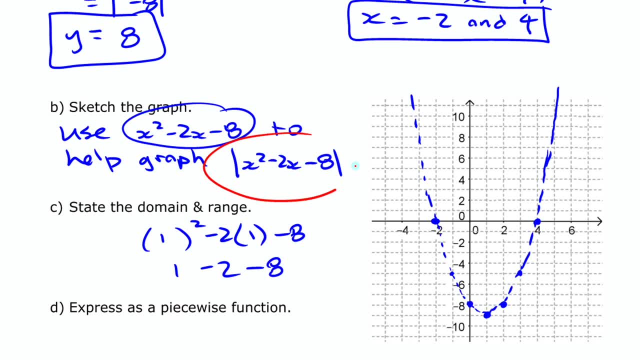 Now, if you want to graph absolute value of that, the absolute value of that is going to be where? anywhere that it already has a positive y value. anywhere where this already has a positive y value is not going to change. So this part above here is not going to change. 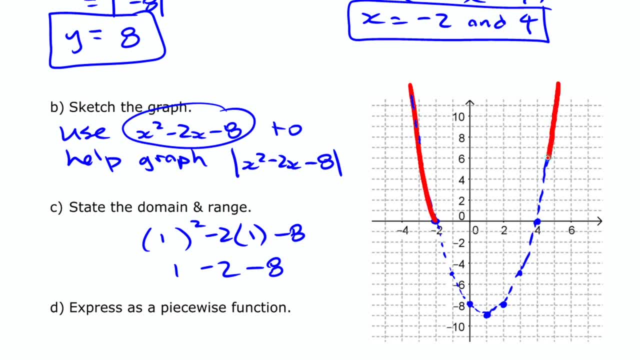 That part's going to be the same And this part's going to be the same, But the parts that have negative y values. so this part down here, The parts that have negative y values, are going to get reflected up above. So this: 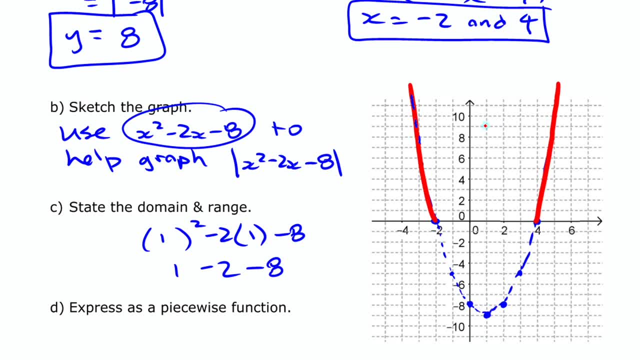 point down here. that vertex is not going to be at negative 9, it's going to be at positive 9.. The intercept, as we saw before, is going to become positive 8 instead of negative 8. And so that point's going to be like that. If you wanted to put those other ones, maybe. 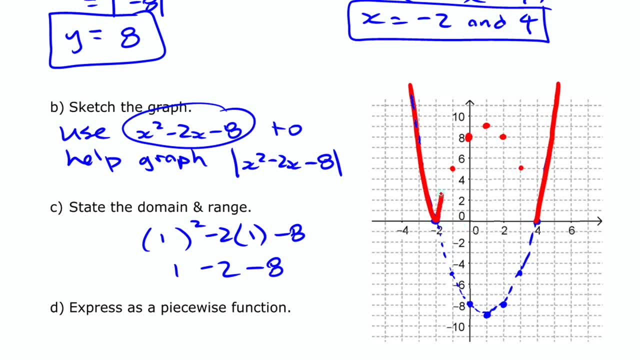 you could put those as well, But that part is going to get reflected up above, So this graph's going to look like this strange w-shaped thing. So what's in red there is this. That part gets reflected up above. If you want to look at the domain and the range, the domain doesn't actually change. 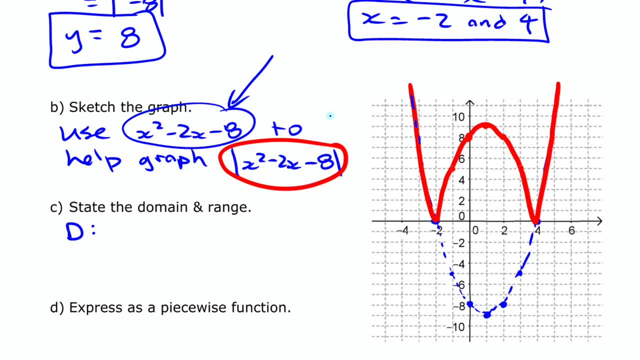 for this: Any x values permitted there, there's no restrictions. The same here: You put any x value there. So this is all real numbers. The thing that changes is the range, Since we reflected all the negative parts up above. the range is just. 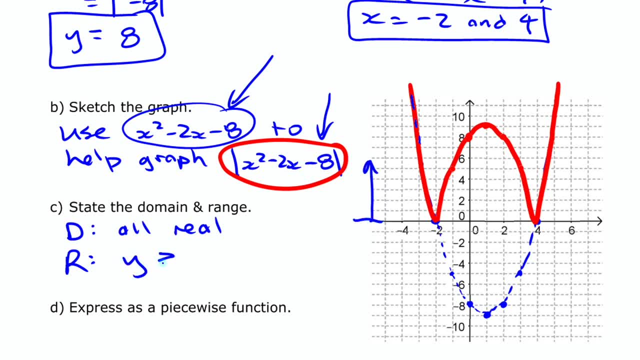 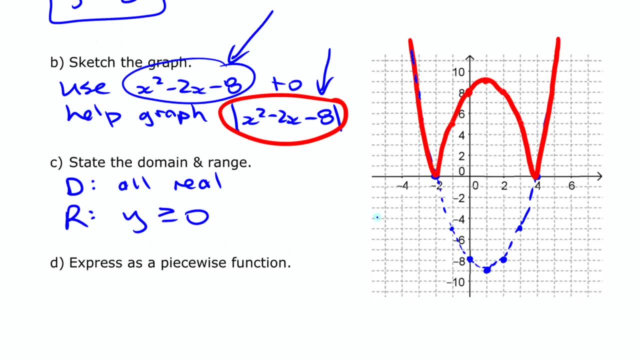 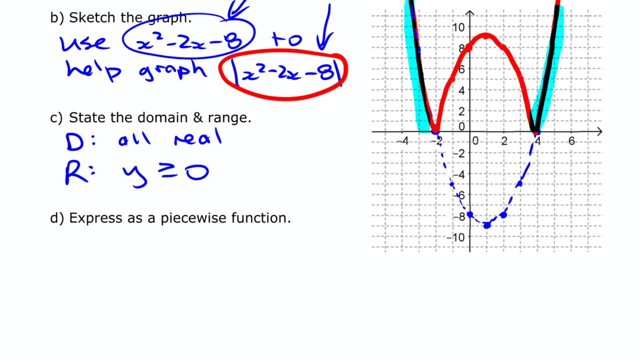 0 and above. So this is: y is greater than or equal to 0, right, There can't be any negative y values. If we're going to write this as a piecewise function, it's just expressing those two different parts of the graph: The part that stayed the same, that didn't change, and then the part 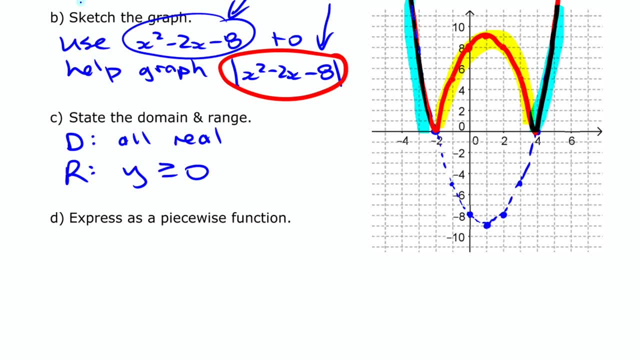 that did get reflected became the opposite. So if we're going to write that, we're going to write: absolute value of x squared minus 2x minus 8 is equal to these two pieces here. It's equal to itself. It didn't change If this is going to be a bit harder to write. 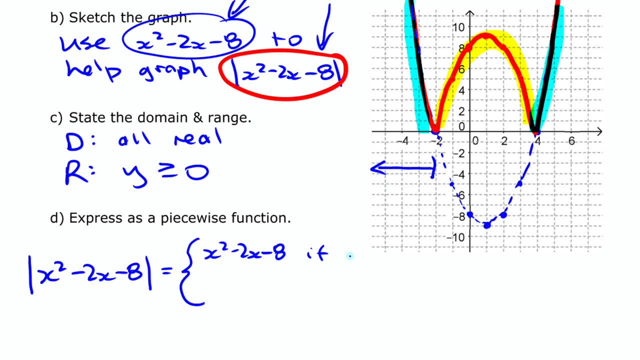 here, but it's if you're less than or equal to negative 2.. So if x is less than or equal to negative 2, or it's greater than or equal to 4.. Or x is greater than or equal to 4.. 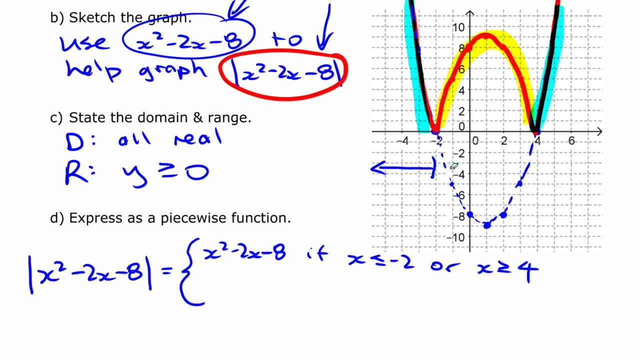 That's the part that didn't change. The part that did change. it became the opposite. So it became the opposite of this. Put a negative in front. That was when you were between negative 2 and 4. So if x is, 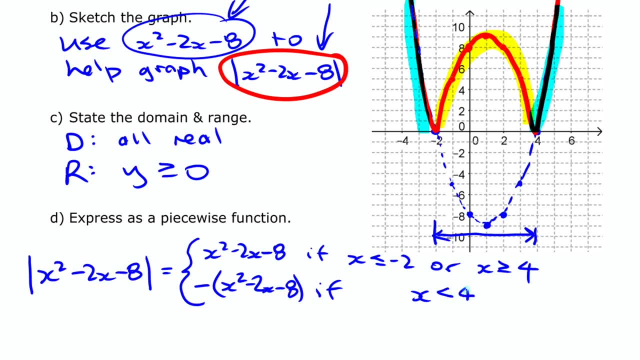 you can write a double inequality here, If x is less than 4 but greater than negative 2. Write that double inequality If both of those conditions are true, If it's greater than negative 2 and less than 4.. Alright, So that's a piecewise function. for that The 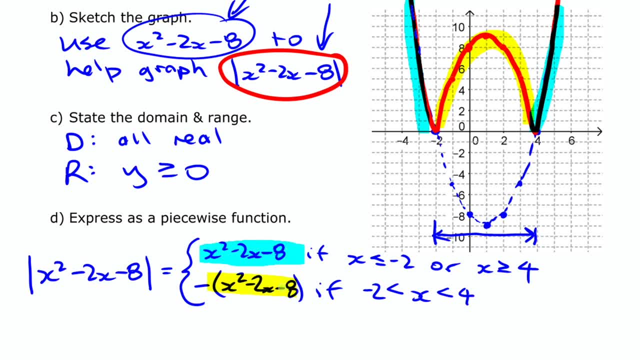 blue part. This part is the blue part that didn't change. This part is the yellow part that did get reflected up above. Alright, As before that yellow part. there you could have written: you could distribute the negative and make it negative: x squared plus. 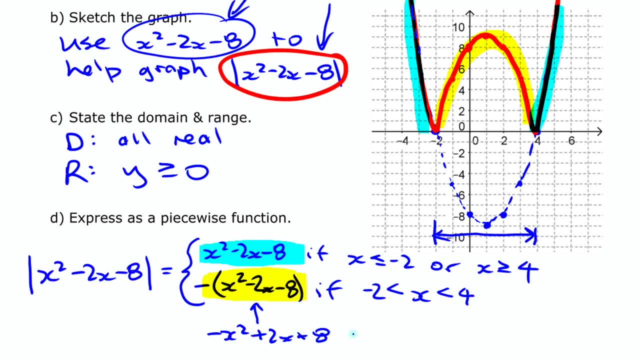 2x plus 8.. Switch all the signs if you want. Alright, so that is a look at the absolute value of a function, where the function you're talking about is a quadratic function. Alright, so we're done.